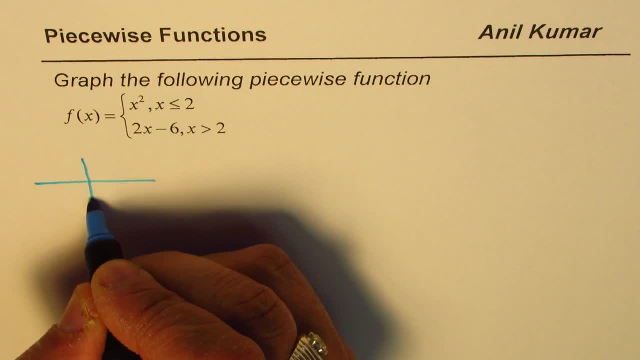 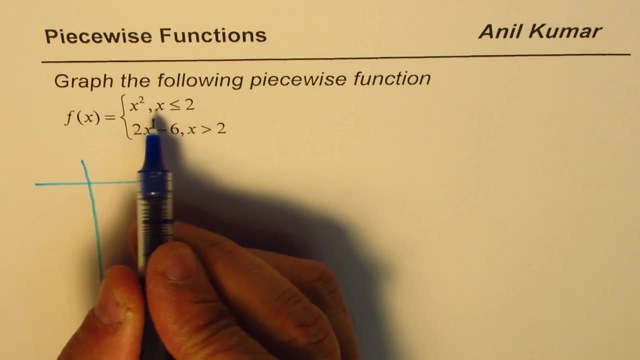 So best way to graph is to make table of values right. So let's make table of values to graph. So the first one is when x is less than 2, right. At that time f of x equals to x square. So f of x. 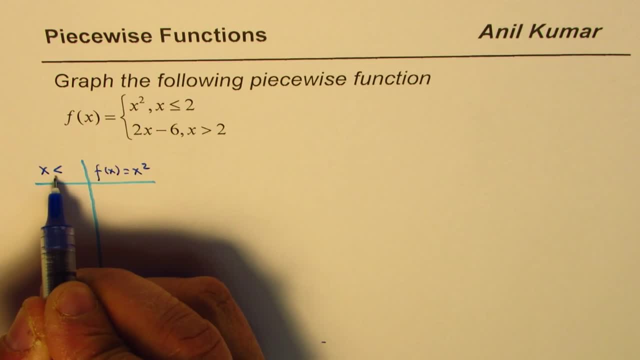 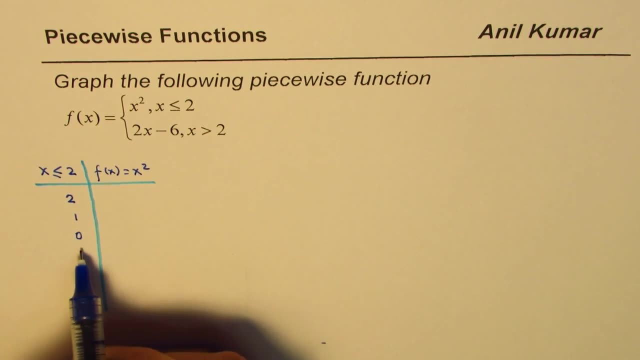 equals to x square when x is less than equal to 2.. So what we can do is we can begin by taking values like 2, 1, 0, minus 1 and 2.. Let's calculate these values using calculator. 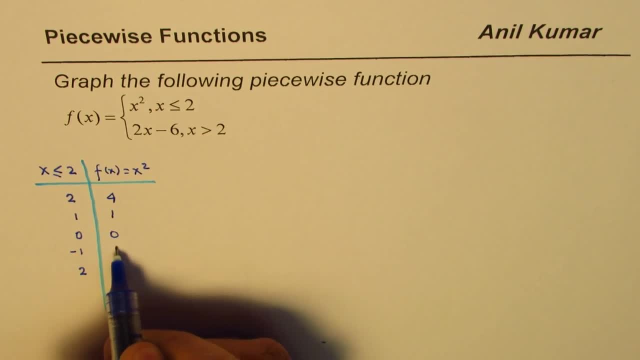 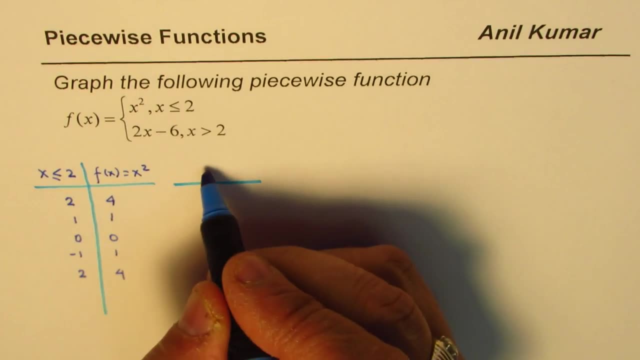 Well, x square, so 2 square is 4, 1 square is 1,, 0,, 1 and 4.. So we get these values. Now let us also sketch what happens when we have x values which are greater than 2.. So now we will do. 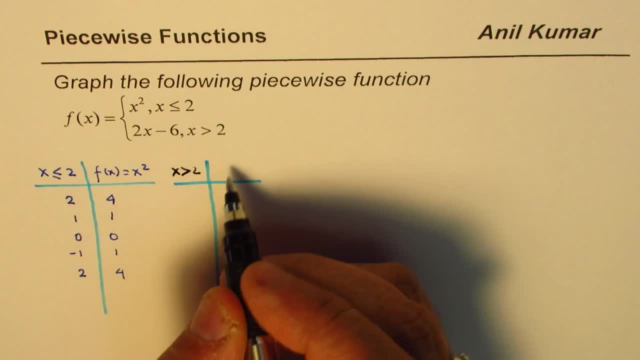 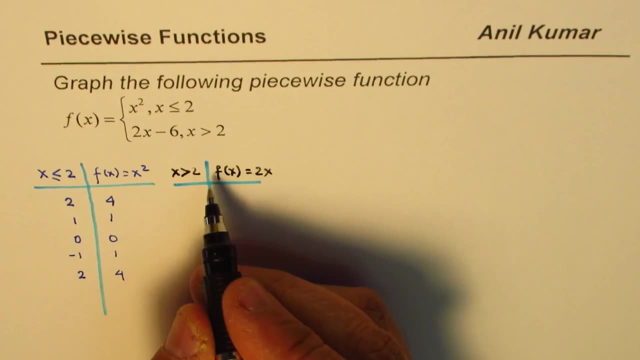 for x greater than 2.. In that case the function f of x is equal to 2x, So greater than 2.. Let's take the value 2 also, and we say it is slightly more than 2.. So I'm just putting that. 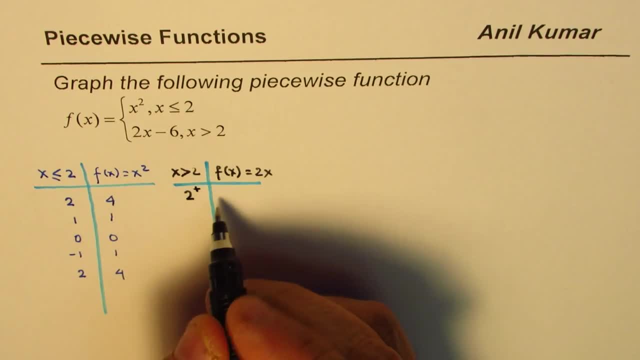 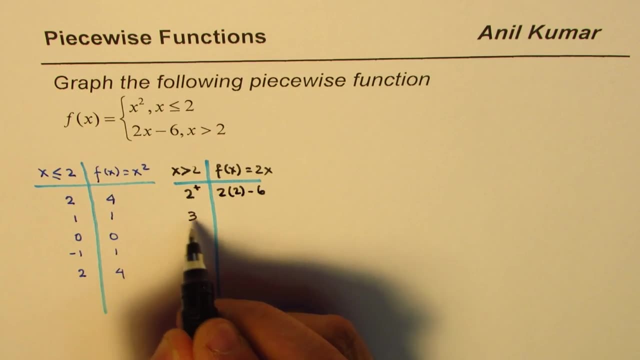 plus here slightly more than 2.. But I'll place 2 here, So we get 2 times 2 minus 6, and then, if I write 3. So we'll write 3 here, 2 times 3 minus 6, and 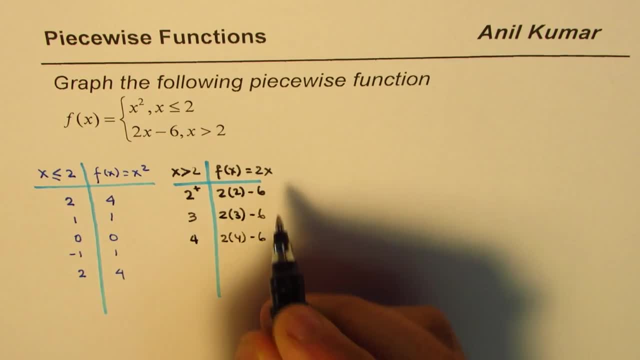 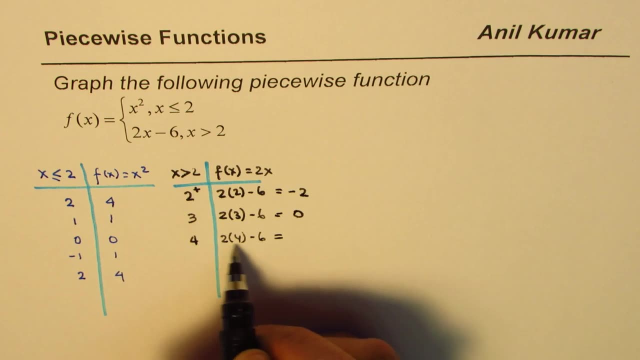 we can write 4.. 2 times 4 minus 6, right? So that gives you: 4 minus 6 is minus 2.. 6 minus 6 is 0, and that is 8 minus 6 is 2.. You could write 2 to the power of 2 times this minus 6, which will be. 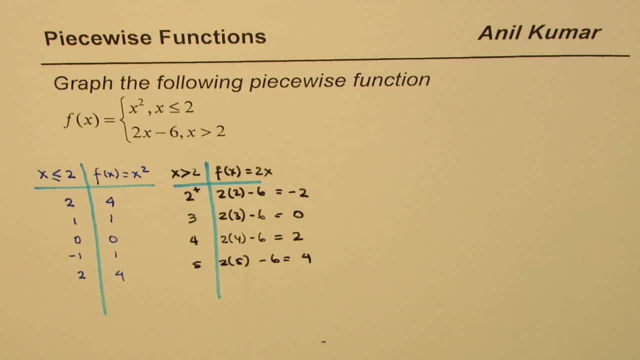 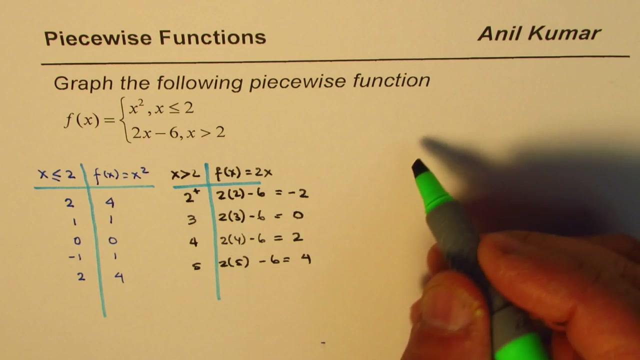 4, right? So these are the values. So once you have the values, you can have a calibrated graph, but we'll do with our approximate one. So let me sketch my graph. So we're looking for some values between, let's say, 2 to 5.. So what? 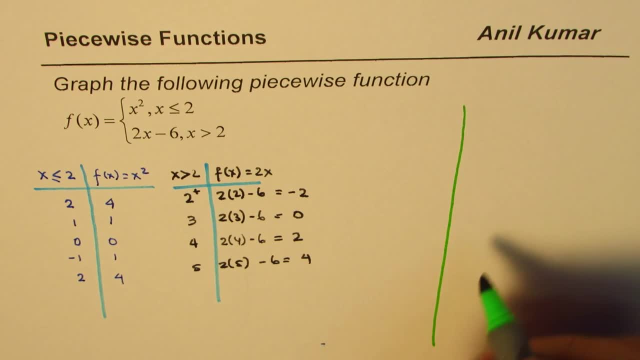 we'll do here is: we'll make more towards the left side And what we have is most of the values are positive for us except for this. So we'll make this. Let's say this is 1, 2, 3,, 4,, 5, 6.. Let's say this is minus 1, minus 2, minus 3.. Okay, this is minus 2.. 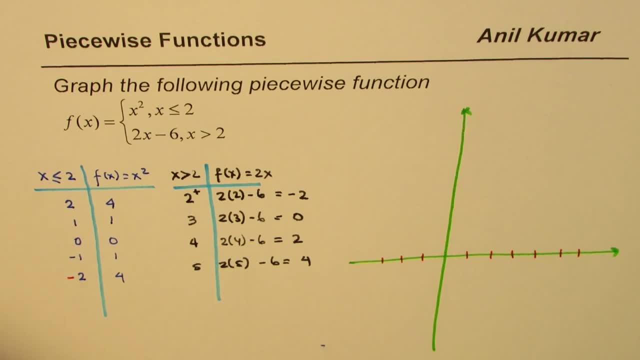 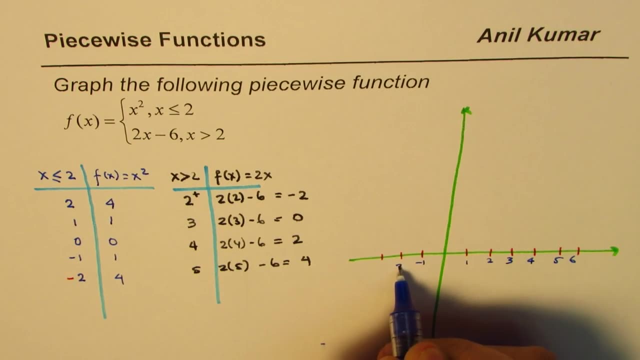 Right. So the values here are 1,, 2,, 3,, 4, 5, 6.. This is minus 1,, minus 2,, minus 3.. That's 0.. And on the y-axis, we are going up to 4.. 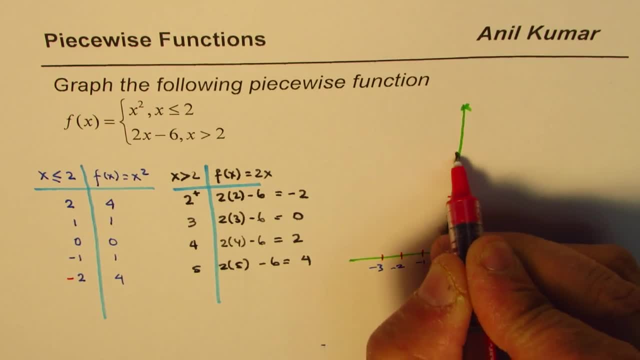 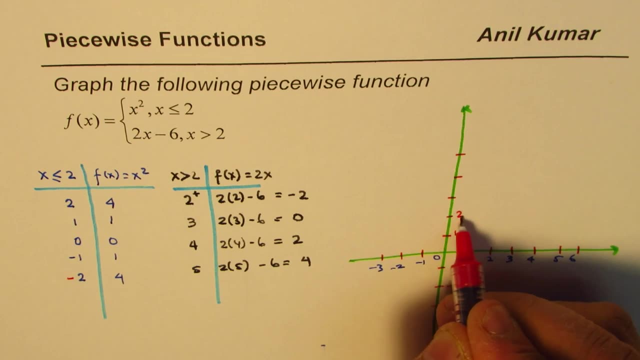 That's okay. So 1,, 2,, 3, 4, 5, minus 1, minus 2, minus 3.. So this is minus 2 for us, and this is 1,, 2,, 3, 4, 5.. 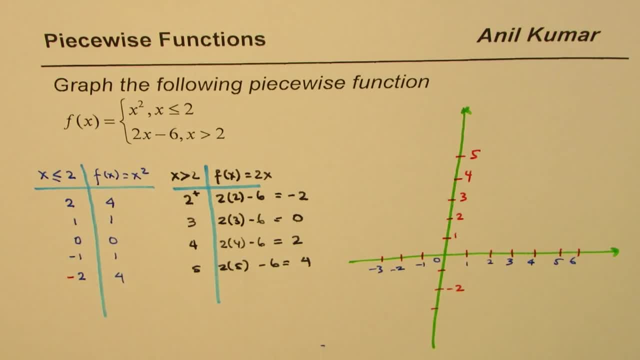 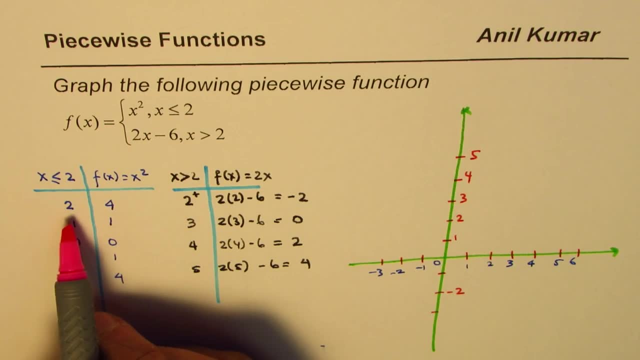 So on the graph let's plot these values. The first one on the left side is for: f equals to x square. So the parabola taking the values from 2.. 2 is equal to 3.. Okay, included here, 2 square is 4, so 2 square is 4. so we get this filled up value and then at 1 it is 1. 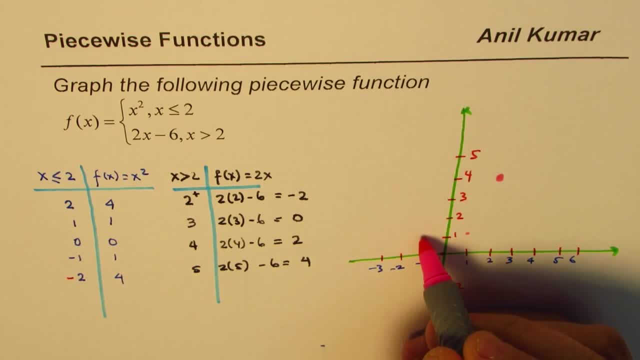 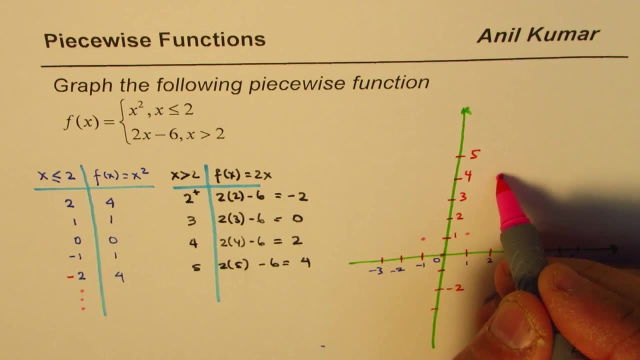 so at 1 it is kind of 1 and then it is 0 and then it is 1. you know it's symmetric right? so the graph is kind of like this. you could have gone like this, and you know how parabolas are. it starts from here. 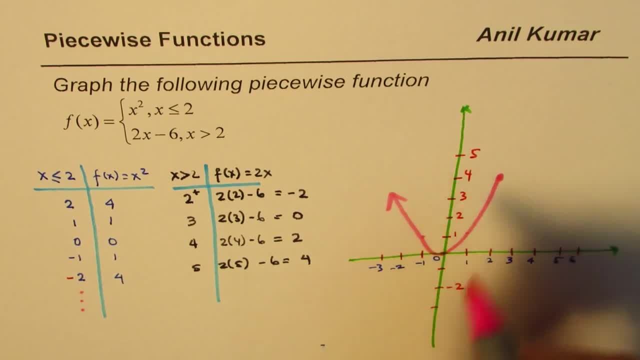 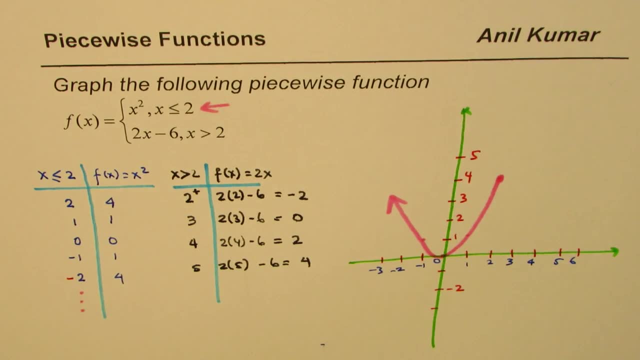 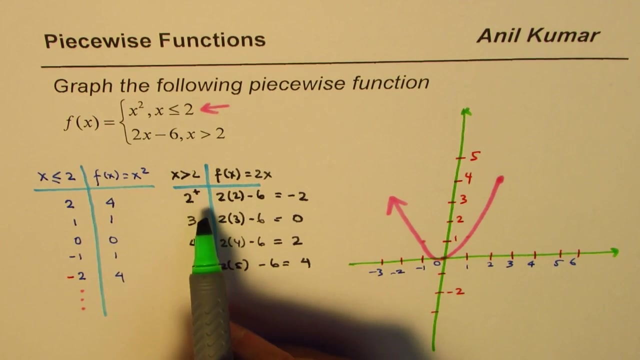 moves downwards, correct, and then you know symmetric about this. we could just sketch like this, so that gives us for less than equal to 2. the other part of the of this graph is a straight line: 2x minus 6. at slightly more than 2, that means at 2 we will have open circle. it is minus 2, so at 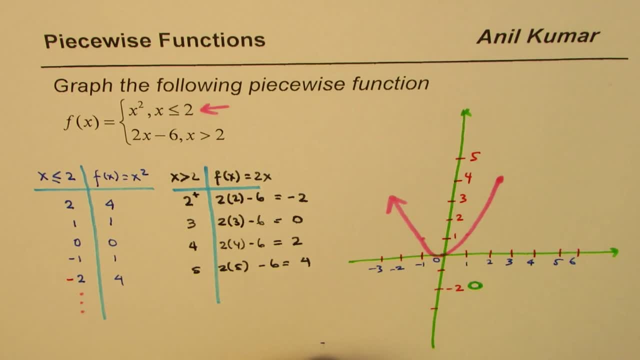 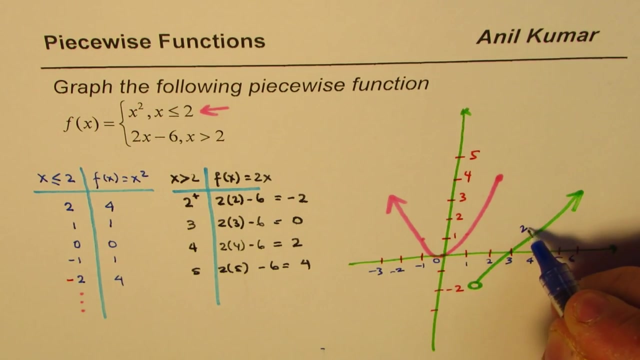 2 it is minus 2, so that is the open circle. right at 3 it is 0, and then it moves on. it's a straight line. so let me just connect it like this, okay, so that becomes the graph. treat the other line as a straight line, which is 2x minus 6, and this: 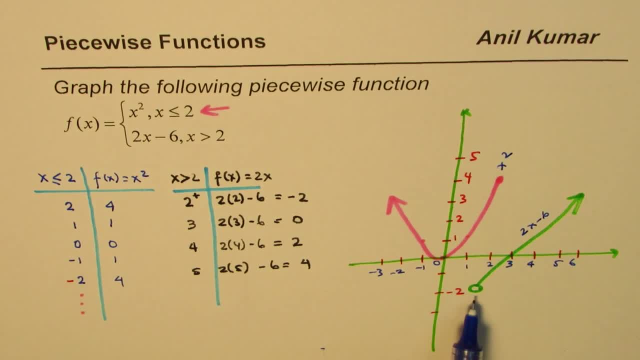 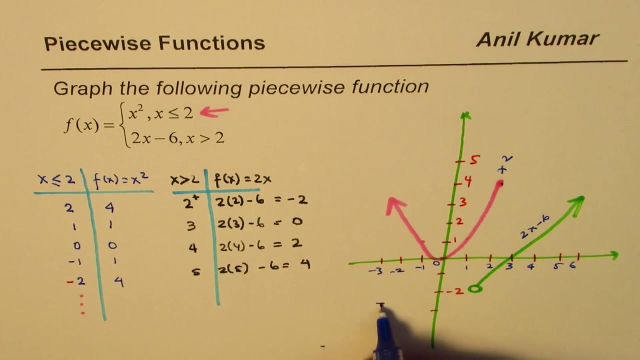 one is x square. so see, this is a filled up. so in this particular piecewise function we have two pieces, one represented by the parabola, the other one by a straight line, and what you observe here is kind of a discontinuity, do you see that? and this discontinuity type is called jump discontinuity. 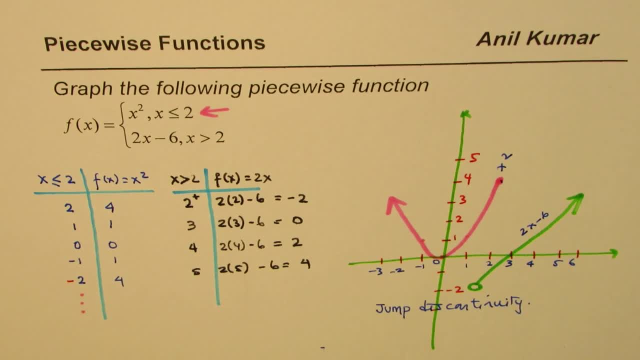 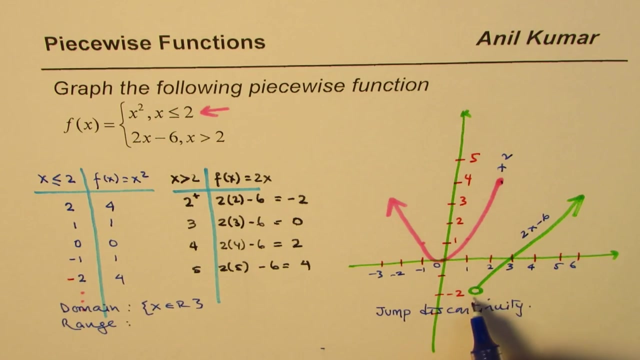 okay, so we have done this. let us also write domain and range of this function. can you write down domain range? let's write domain is what? so domain of this function is, since we have some values. at 2, therefore, the domain is x, belongs to real numbers. how about range? range of this function. 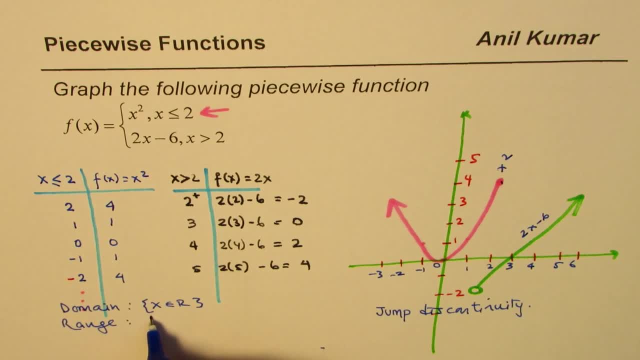 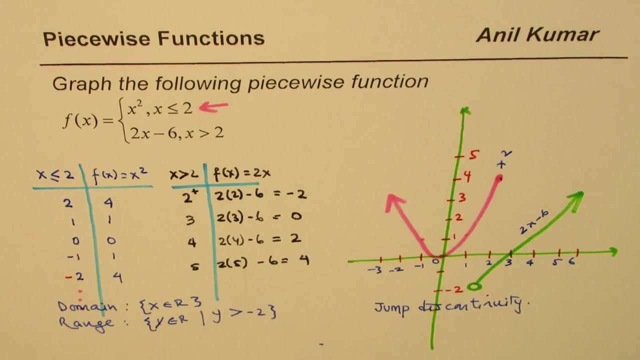 is always greater than minus 2, right? so it's y belongs to real numbers where y is greater than minus 2. so note: it is not equal to minus 2, right? but anyway, in this video we have learned a very important technique, and that is to graph. 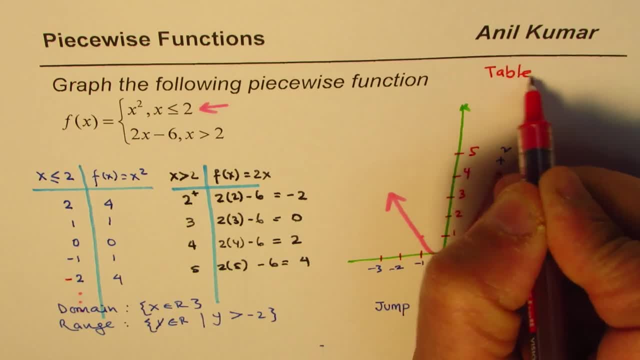 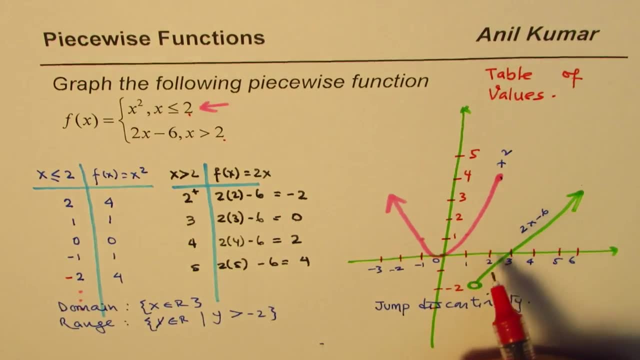 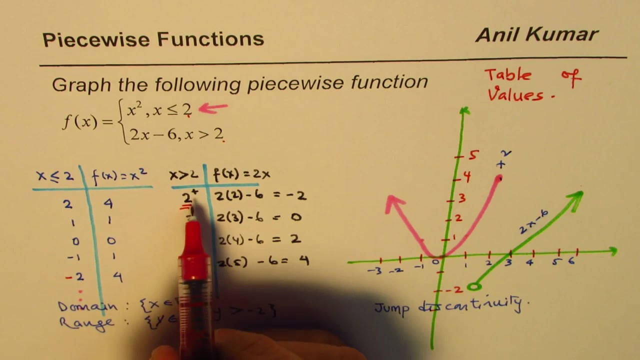 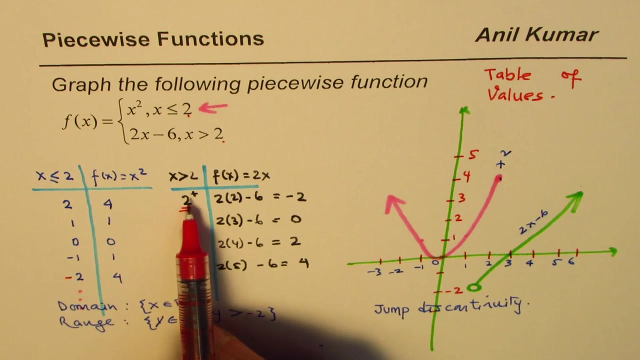 piecewise function. it is good to have table of values. they help, and it is very important to analyze the point where the graph switches over from one piece to another. so i use this kind of plus to indicate that we are now working on the second piece. right, but it's important to check the starting point, which can be 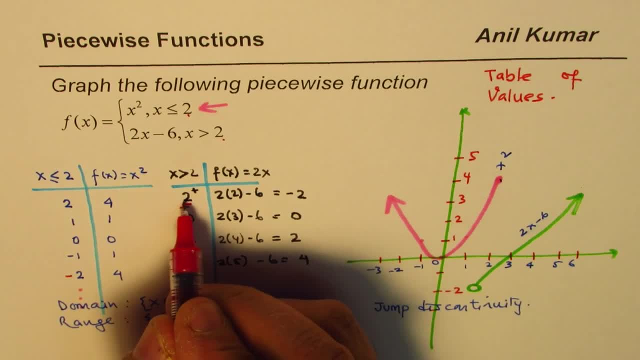 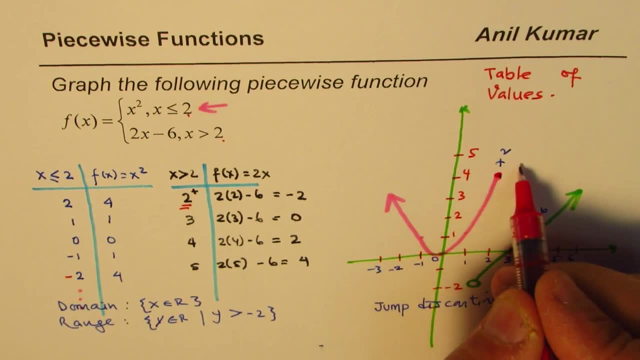 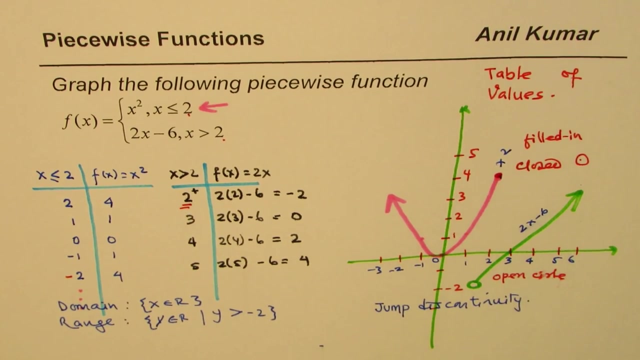 shown as open circle. so this point here is shown as open circle. that means not included. this one is closed circle or filled in circle. do you see that? so that is how we should be sketching piecewise functions. i am andal kumar and i hope all this is absolutely. 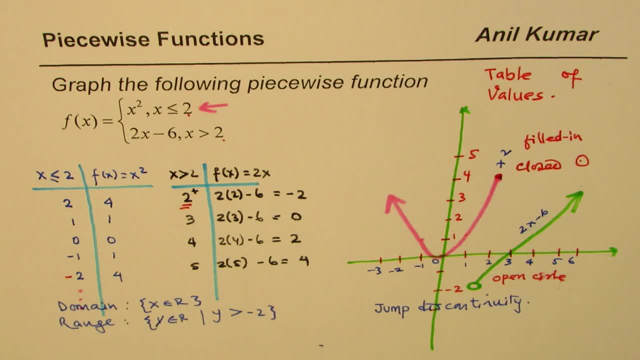 clear. if you have questions, please feel free to post them. thank you and all the best.